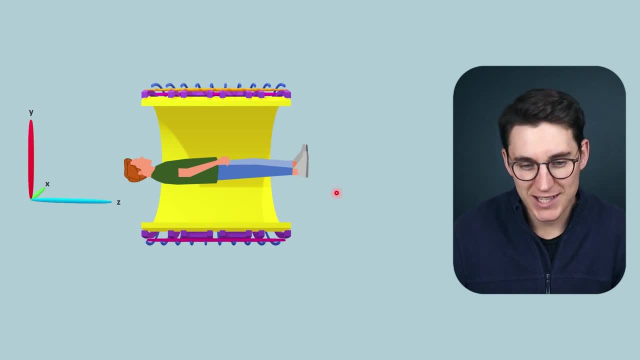 we use is what's known as the Cartesian plane. We can separate this image into three separate axes. The first, by convention, is the longitudinal axis, the axis that runs from head to toe along the patient, and that's always the longitudinal axis. The longitudinal axis is the axis that runs from head to toe along the patient, and that's always. 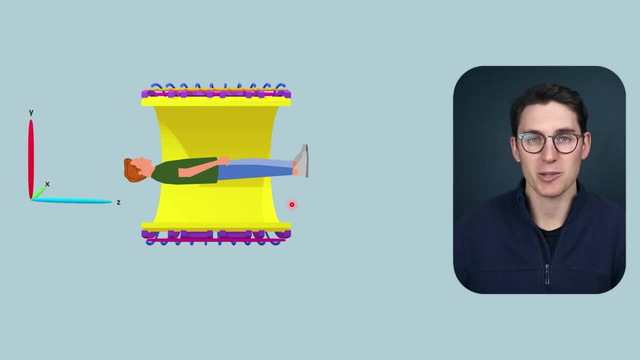 labeled the Z or Z axis. We can then cut the patient in transverse section axial plane using the XY axis here or the XY plane, and that's what's known as the transverse plane. So we've got the longitudinal plane and the transverse plane, and these are really important concepts to take. 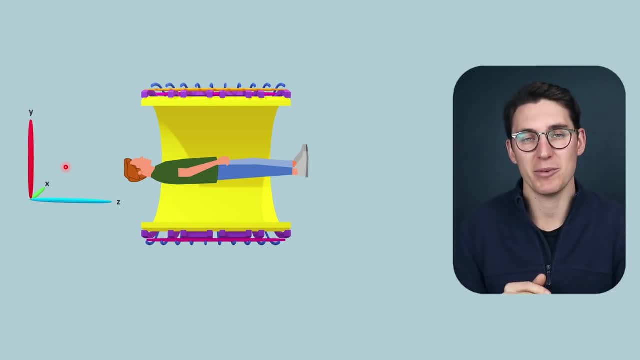 forward into the upcoming talks. Now, in MRI imaging, we use a concept known as nuclear magnetic resonance. We use a large magnetic field in order to induce resonance- certain atoms- within the patient, and in MRI imaging we use the hydrogen atom to do this. Now, the hydrogen atom is useful one because it's abundant within the 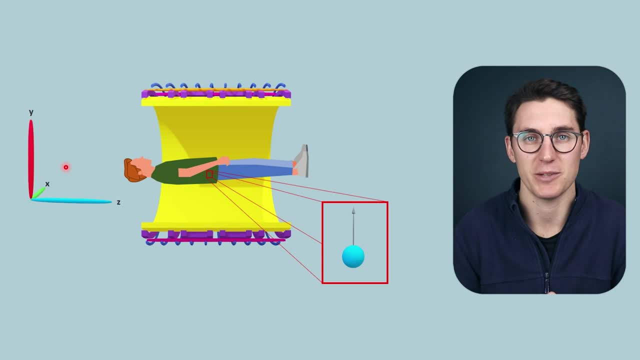 body. there are billions of hydrogen atoms within the human body and two. the hydrogen atom has what's known as nonzero spin, and atoms with nonzero spin effectively act as tiny bar magnets within the body. they have a north and a south pole and, as a result, have what's known as a magnetic moment. Now the 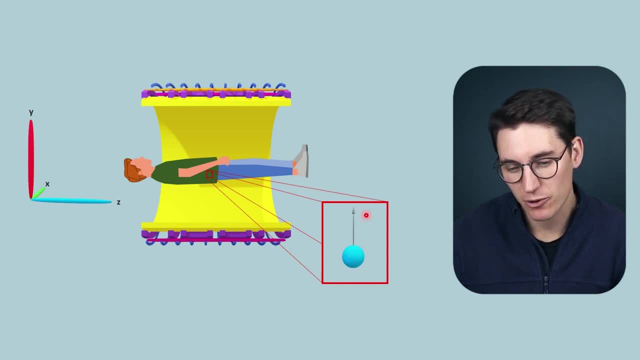 magnetic moment in these diagrams is represented by this arrow here. Now the arrow can actually be used as a vector within the MRI machine. it has both direction and magnitude, and the combination of the magnetic moments amongst all the free hydrogen atoms within the body is what's used to. 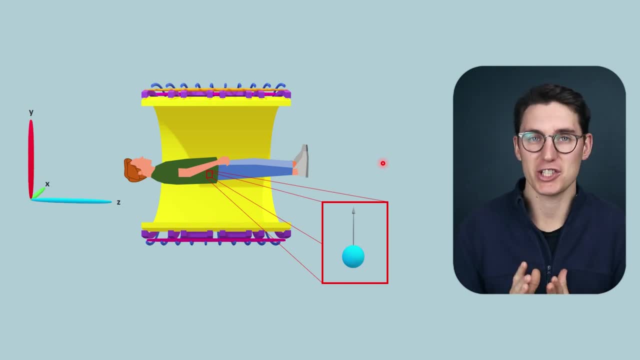 generate the image. Now, in conventional MRI imaging we only use the hydrogen atom to create our MRI imaging, so we can think of our patient as being a combination of multiple different hydrogen atoms that are moving randomly within the body, moving with Brownian motion, and the amount of movement is determined by the 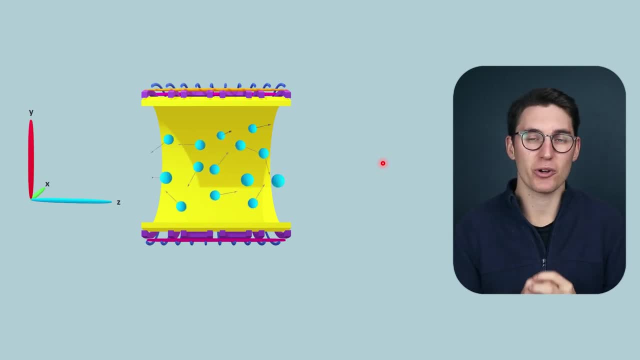 temperature of that patient. Now, because hydrogen protons have a magnetic moment, they will be influenced by an external magnetic field. much like a compass aligns with the magnetic field of the Earth's core, we can also pass a large magnetic field across the patient. That magnetic field will cause two. 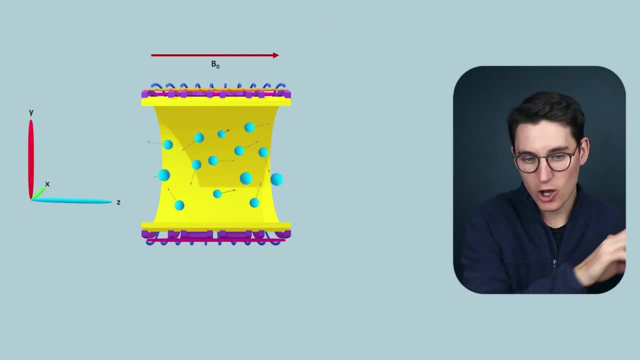 things to happen. the first is that the hydrogen atoms will align with the magnetic field and the second is that they will precess around their own axis. If you think of a spinning top on a table experiencing gravity, the spinning top precesses, like this, around its own axis. 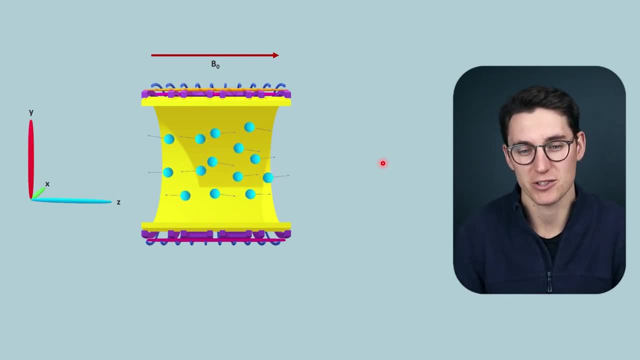 the same thing is happening to these hydrogen atoms within the patient. They are along the main magnetic field of our MRI scanner and they precess at a certain frequency. Now that frequency is determined by the type of atom. so here it's hydrogen and it's determined by the strength of the magnetic field. 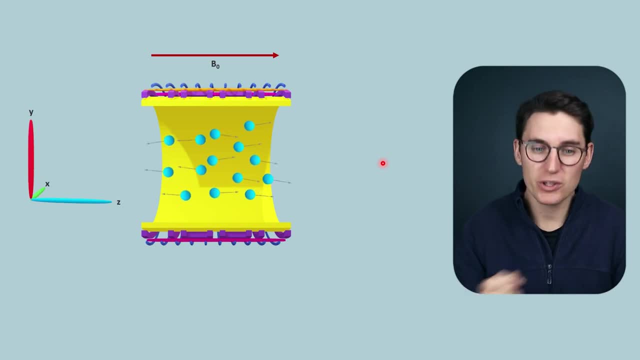 The precession frequency is directly proportional to the strength of that magnetic field. The higher the magnetic field, the higher the precessional frequency. Now, don't worry if this is starting to confuse you. We're going to look at each one of these factors in isolation in the coming talks. 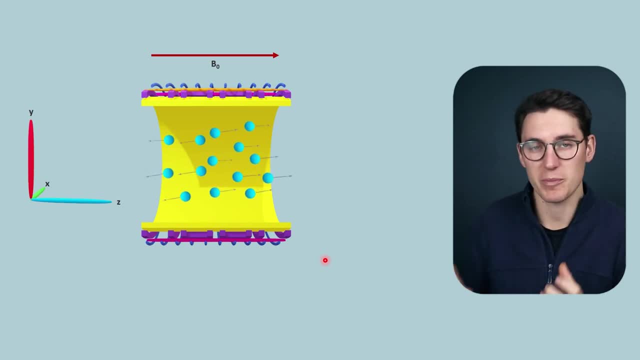 Now, as you can see, the hydrogen atoms either align parallel to the magnetic field or anti-parallel to the magnetic field, And in fact, when we look at quantum physics later, the hydrogen atom itself exists in both of these states. But for now what's important is that the absolute number of hydrogen atoms 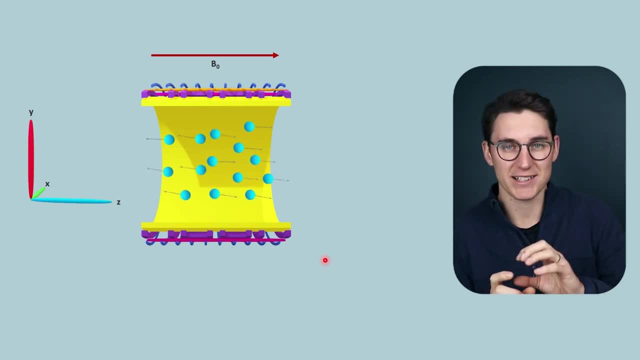 that exist in the parallel direction exceed those of that in the anti-parallel direction, And those in the parallel direction are in a slightly lower energy state to those in the anti-parallel direction. Now we can combine these magnetic moments to create a net magnetic moment. 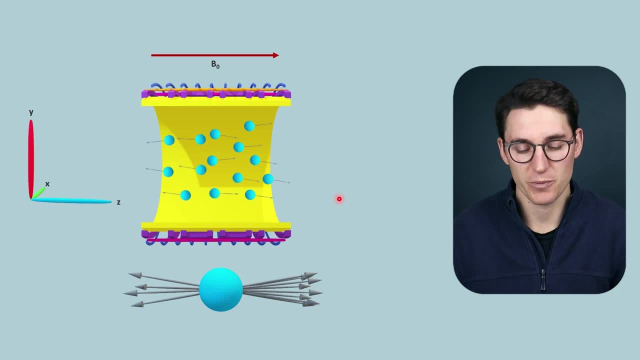 within the sample that we are applying this magnetism And, as you can see, there are more magnetic moments in the parallel direction than there are in the anti-parallel direction. Secondly, to note, although the hydrogen atoms are precessing at the same frequency, 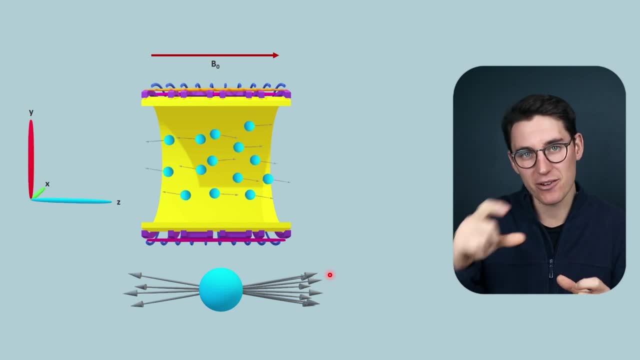 they are out of phase from one another. The x and y vectors on each individual magnetic moment here cancel each other out. You can see there's an equal distribution within the x and y plane And what we get here is what's known as net magnetization vector. 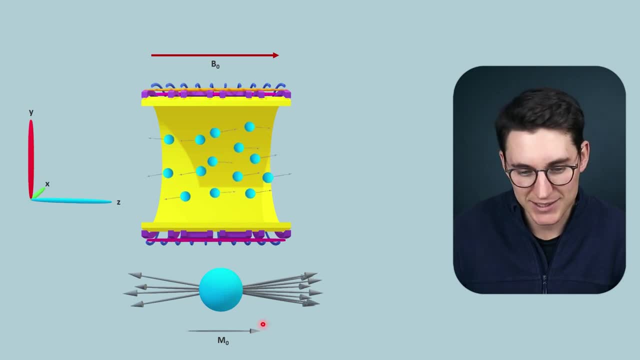 We combine all of these magnetic moments here and we get the net magnetization vector. Now the net magnetization vector is along the longitudinal axis, the z-axis on the Cartesian plane. There is no x or y value here because those precessional frequencies. 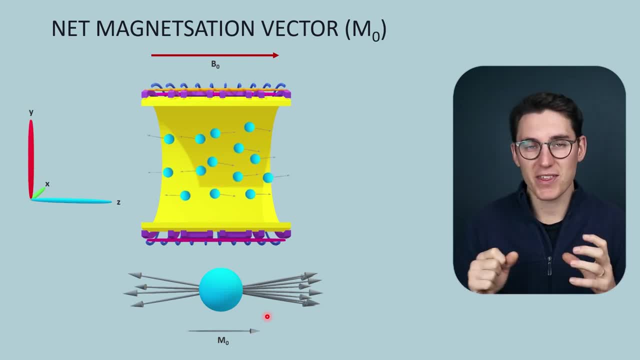 are out of phase with one another. Now we mustn't think of individual hydrogen atoms when we are looking at MRI imaging. We need to think of the net magnetization vector and how that is influenced by changing magnetic fields within the MRI machine. 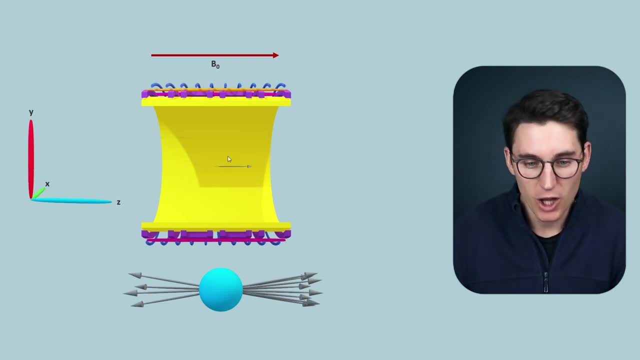 So what we can do is replace these hydrogen atoms with the net magnetization vector. here Now, within MRI imaging, what we want to measure is this net magnetization vector, but we can't measure it along the parallel direction, along the longitudinal direction here. 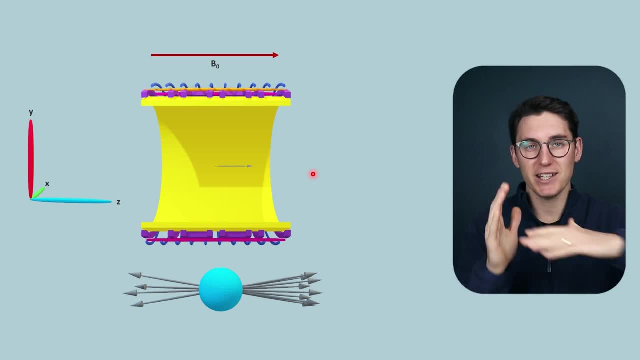 because our main magnetic field strength is too strong and it will interfere with our measurement of this net magnetization vector. What we want to do is move that net magnetization vector perpendicular to our main magnetic field. That will allow us to measure that signal and that's exactly what we do in MRI imaging. 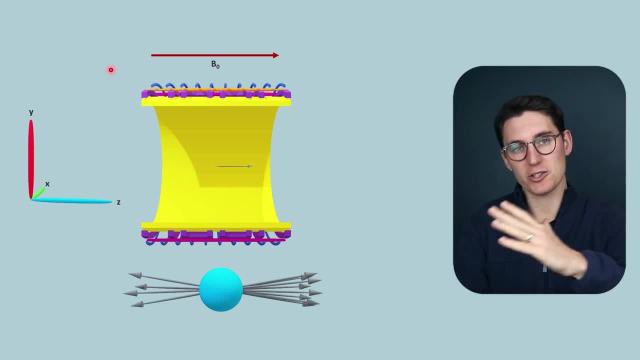 We have our main magnetic field that is forcing those protons into the parallel direction. What we then do is apply a second magnetic field known as the radio frequency pulse. Now the radio frequency pulse acts in the perpendicular plane to that main magnetic field and the radio frequency pulse 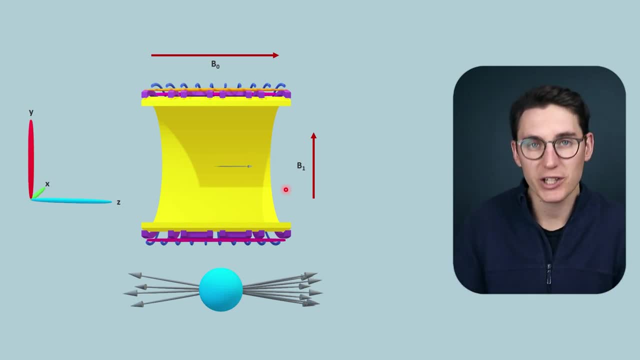 alternates at a frequency that is equal to the precessional frequency of the protons. If the frequency of the radio frequency pulse matches that of the precessional frequency of the hydrogen atoms within the patient, two things will happen. The first is that the protons will start to fan out and become more perpendicular with the main magnetic field. 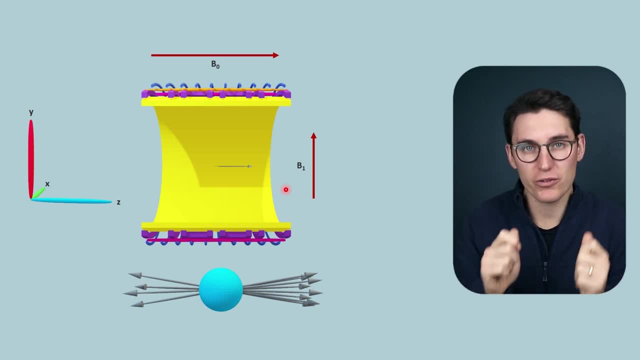 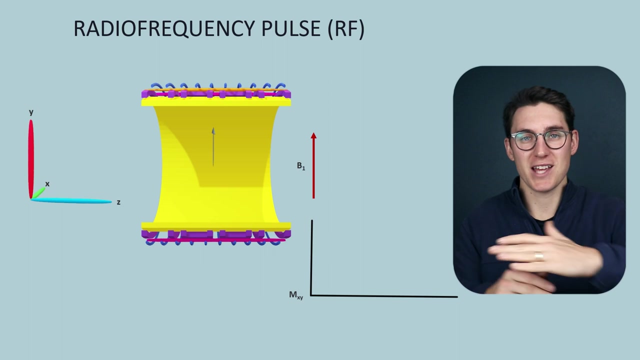 And the second is that the precessional frequencies of those protons will start to precess in phase. Our net magnetization vector now will get some transverse magnetization, some magnetization in the x-y plane. So as we apply this radio frequency pulse, that net magnetization vector will start gaining some transverse magnetization. 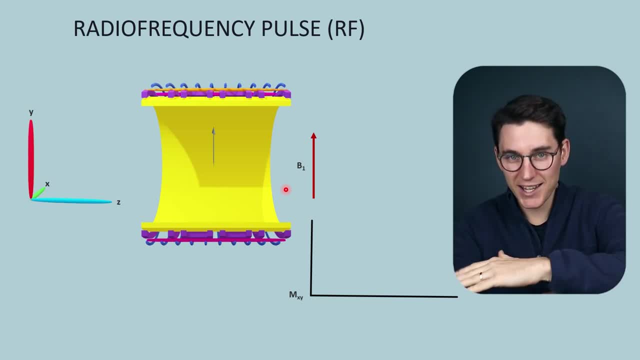 And the angle at which we flip that net magnetization vector is what's known as the flip angle. In this example we flipped it 90 degrees here. Now the protons are all precessing in phase with one another and they now lie 90 degrees. 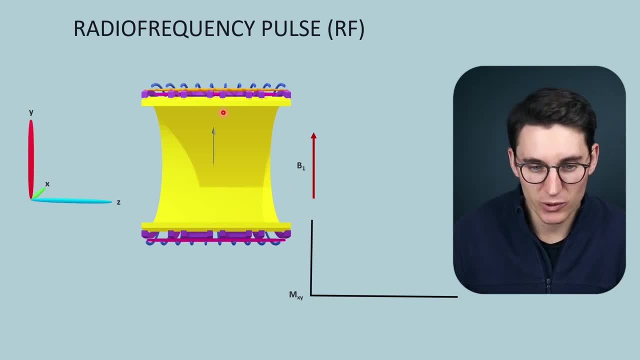 to the main magnetic field. Now what we can do is place a small coil here and the movement of a magnet- as we've seen with Faraday's law of induction, the movement of a magnet can induce a current, And it's the movement of this net magnetization vector that induces a current within our receiver coil that we then use. 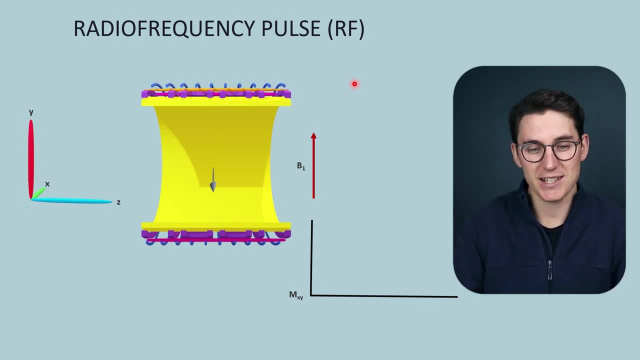 that signal to generate our image. So we can see this now: vector precessing in the transverse plane, in the x-y plane, And we can measure a signal based on the movement of that vector within the transverse plane. Now this vector is only moving in this plane because of that radio frequency pulse. 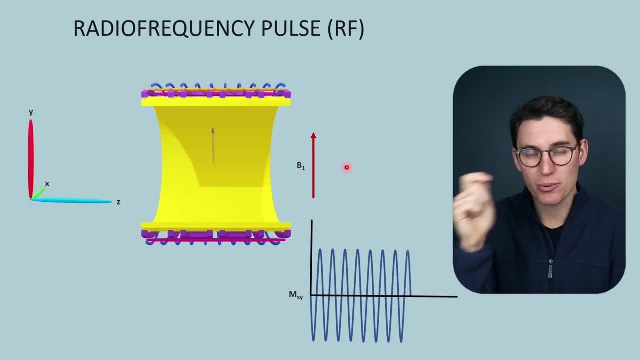 And, importantly, that radio frequency pulse has to match the precessional frequency of the hydrogen atoms. If you're jumping on a trampoline and someone is jumping at exactly the same time as you, you will get double bounce, You will get extra energy and you will jump higher and higher. 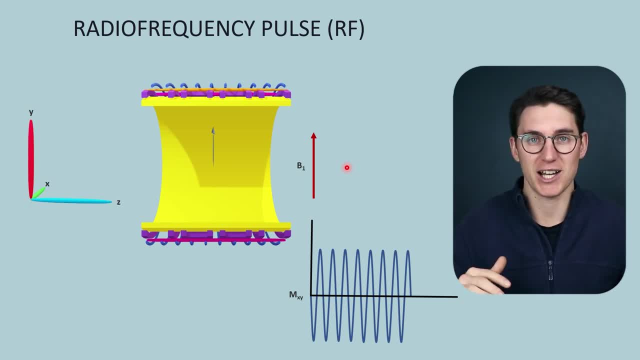 If other people are jumping on that trampoline, but not at the same time, they're not getting that extra energy, They're bouncing the same. Only when those frequencies match will that energy be transferred. Those protons start to precess in phase and the angle of magnetization will start changing. 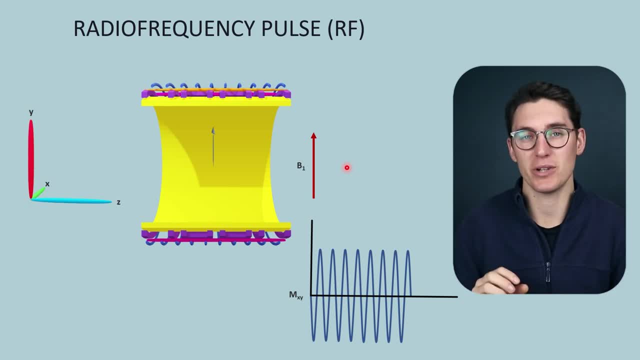 And that angle change is dependent on the time of the radio frequency pulse as well as the amplitude of that radio frequency pulse. Now that we've moved that vector into the transverse plane and we've generated a signal, we want to stop this radio frequency pulse. 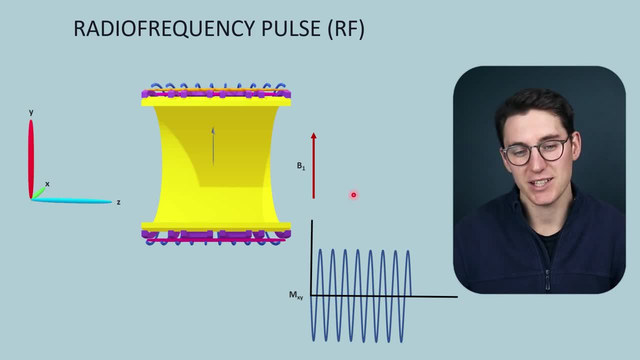 Now we can see, the signal that has been generated here is based on that net magnetization vector precessing at the frequency of the radio frequency pulse. Now we don't actually get a signal like this, because what we actually do is apply a radio frequency pulse and then stop that radio frequency pulse. 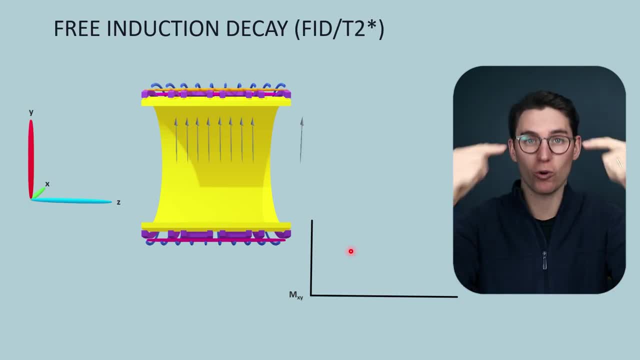 Now what actually happens is the net magnetization vectors are all precessing at that radio frequency pulse And when we stop the radio frequency pulse they will start to go up, They will start to go out of phase again, And it's that loss of phase coherence that will cause a net magnetization vector in the transverse plane to get smaller and smaller. 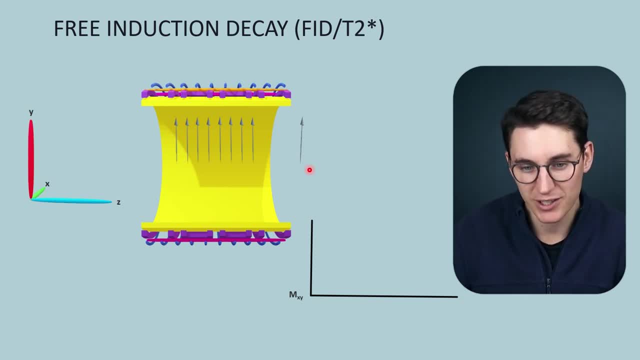 So let's have a look at an example here Here. this arrow here represents the net magnetization vector in the transverse plane. As we stop that radio frequency pulse, we will see the various net magnetization vectors start to become out of phase with one another. 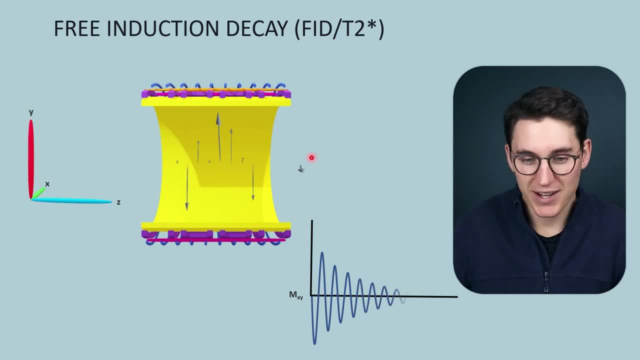 The more and more out of phase they become. The more and more out of phase they become, the less our net magnetization vector in the transverse plane will be, And we see that the signal that is generated becomes less and less. Now, this curve that we draw down like that is what's known as the free induction decayed curve or the T2 star curve. 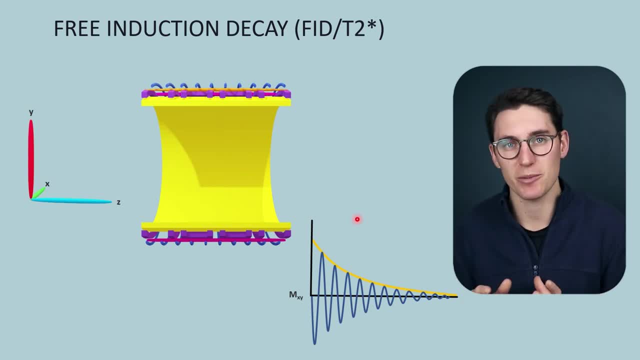 Now, importantly, each and every tissue within the body will have different T2 star curves or different free induction decay curves. If we look at water, the free induction decay is very slow over time, And if we look at something like bone or fat, the free induction decay is much faster. 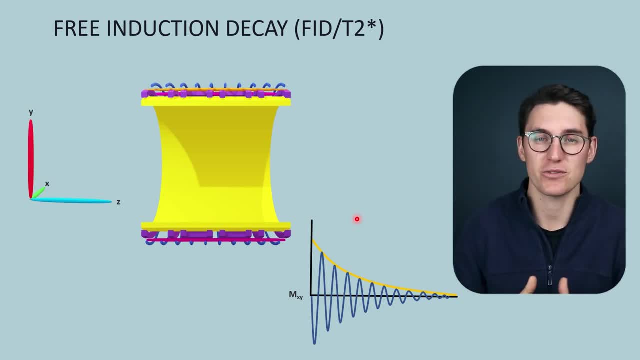 And it's those differences in loss of transverse magnetization that we can use to start generating contrast within our image, And we're going to look at that more within this talk. Now this process is happening simultaneously with a separate, independent process: The loss of transverse magnetization, the loss of the vector within the XY plane. 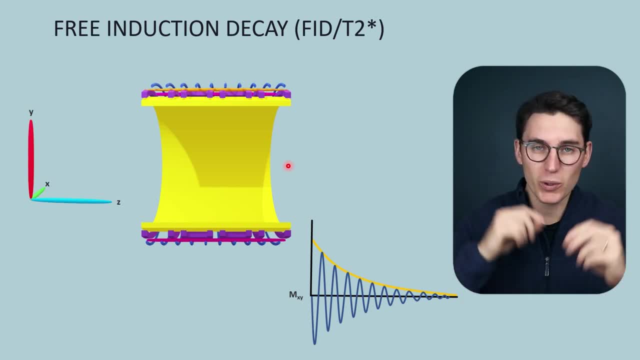 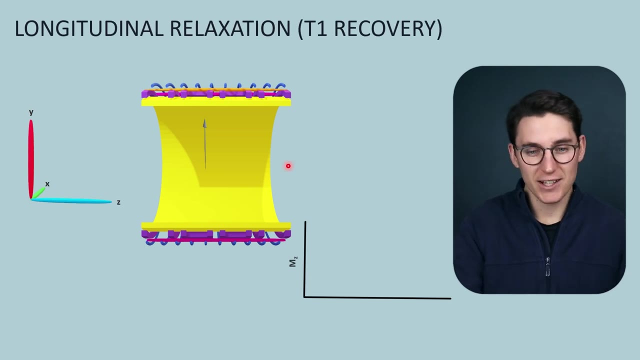 is purely because of that loss of phase between the cells, That is, between the separate protons within the various different tissues. And the rate at which we lose that transverse magnetization is what's known as free induction decay. Now, at the same time, we are also gaining or regaining the longitudinal magnetization within our sample. 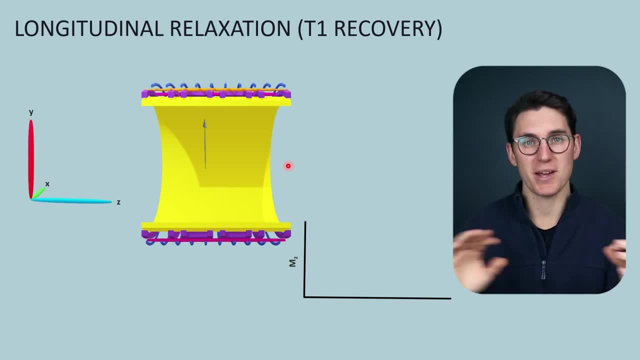 If we have the net magnetization vector perpendicular to our main magnetic field, we have lost all of the longitudinal magnetization or the net magnetization in the Z axis As time goes by and that radio frequency pulse has been turned off. what will happen is that net magnetization vector will slowly regain longitudinal magnetization. 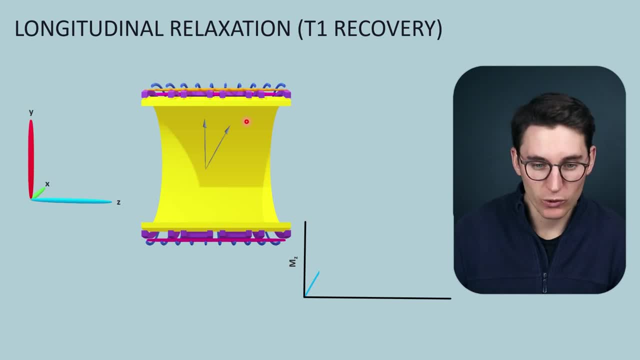 So we can see now, as time goes by, we will regain some longitudinal magnetization. The Y axis here is representing the amount of MZ, or longitudinal magnetization along the Z axis of our Cartesian plane, along the longitudinal axis of the patient. 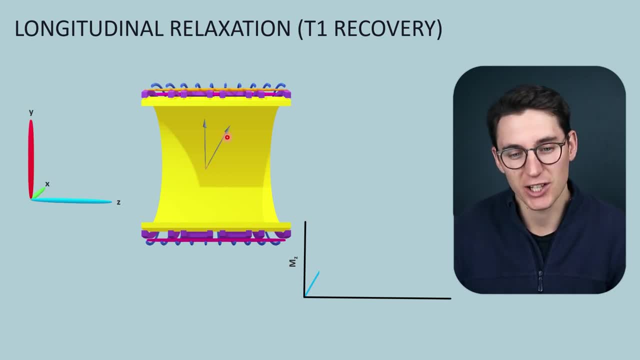 Now, importantly, as we're gaining longitudinal magnetization here, we are not losing transverse magnetization because of the tilt of the protons. We lose transverse magnetization because of those protons going out of phase with one another, That free induction, decay or T2 star. the loss of transverse magnetization. 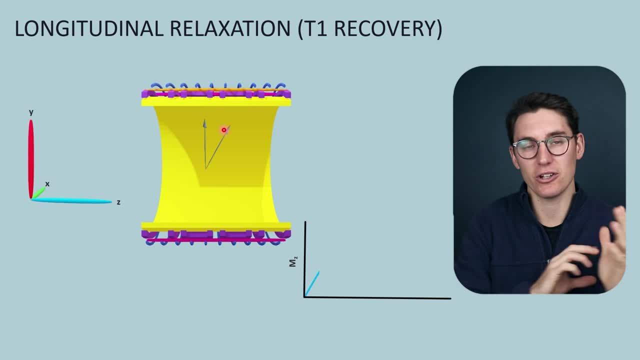 happens much quicker than this. regaining of the longitudinal magnetization. Now, as time goes by, even further, we get more and more longitudinal magnetization. Now, as we can see here, we are gaining longitudinal magnetization, but by this point we have lost all of our transverse magnetization. 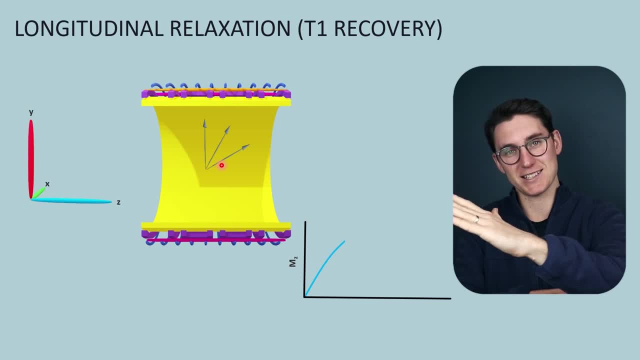 because, although the protons have regained some longitudinal magnetization, by this point they are completely out of phase with one another and all of those XY vectors have cancelled one another out. We are still now regaining longitudinal relaxation, or T1 recovery along the Z axis. 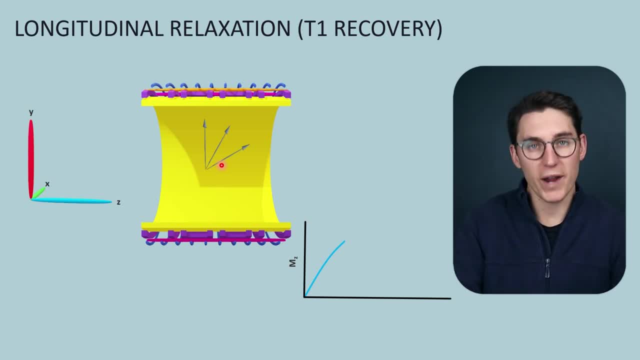 which takes a much longer period of time. Now, when the vectors are all aligned with the magnetic field, with the main magnetic field, we have regained 100% of our longitudinal relaxation. Now important to note that these two processes happen independently of one another. 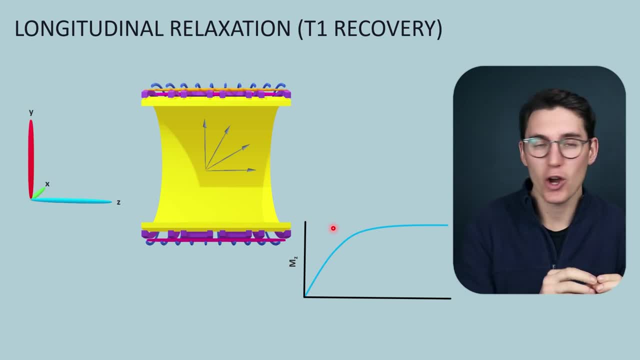 If we know the free induction decay of a certain tissue, we can't calculate the T1 recovery or the longitudinal recovery of that tissue. They are completely independent of one another, Both longitudinal relaxation, like we can see here, and free induction decay. 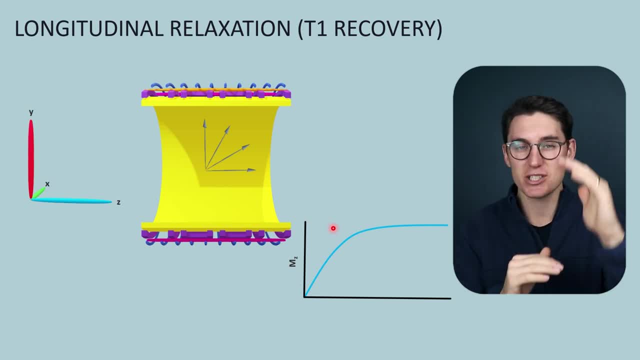 happen at different rates for different tissues, and it's those differing rates that we use to generate contrast within our image. And lastly, and what's most important to remember is we can only measure signal that is perpendicular to the main magnetic field. 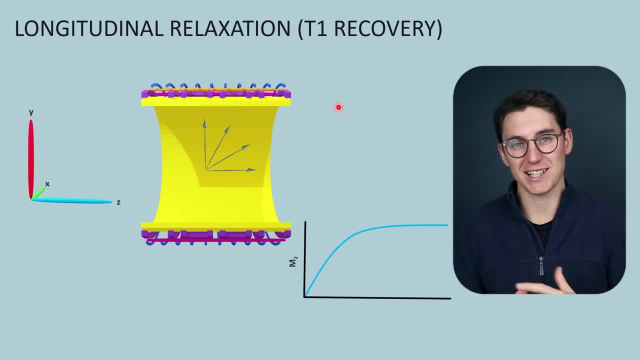 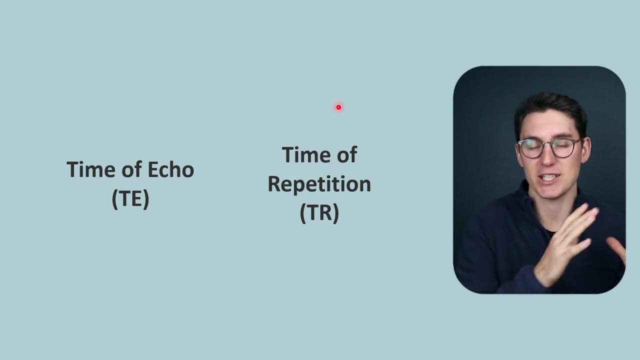 So it's very difficult to measure longitudinal magnetization unless we flip that vector again perpendicular to the main magnetic field. Now we can go about generating images by using two separate parameters that will exploit these differences in the free induction decay, or T2 star decay. 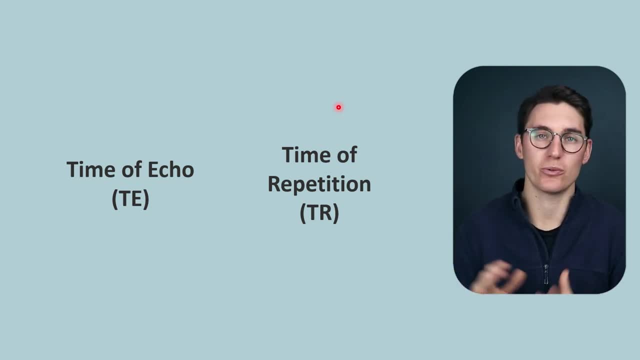 and T1 recovery or longitudinal relaxation. Now the first parameter that we can use is what's known as the time of echo. Now I'm going to use these two knitting needles to show two separate types of tissue. Now we have the protons have been flipped into the longitudinal field. 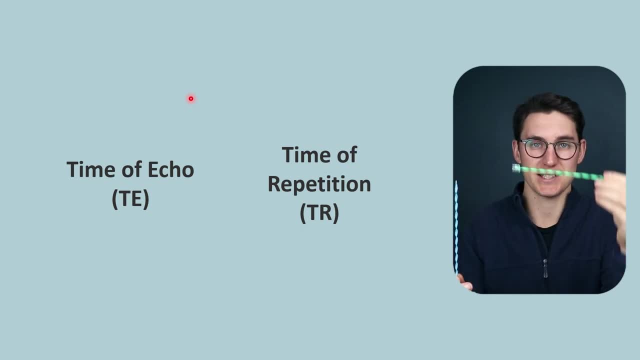 into the longitudinal direction in both of these tissues, say CSF and fat. Now what happens is we apply the radio frequency pulse to 90 degrees. Our protons are now precessing perpendicular to the main magnetic field at 90 degrees. 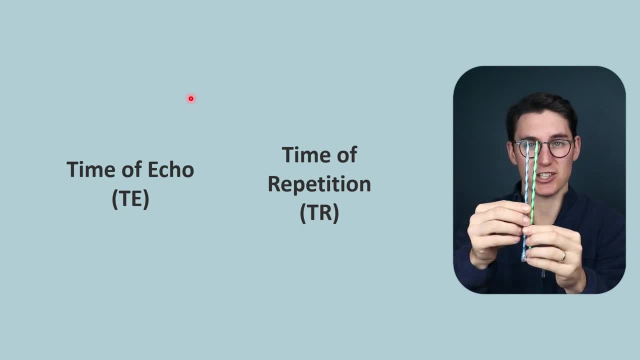 Now what happens is we start to lose transverse magnetization as these start to precess out of phase with one another. We lose that T2, or that free induction decay because these are becoming out of phase with one another. They were initially in phase providing maximum signal. 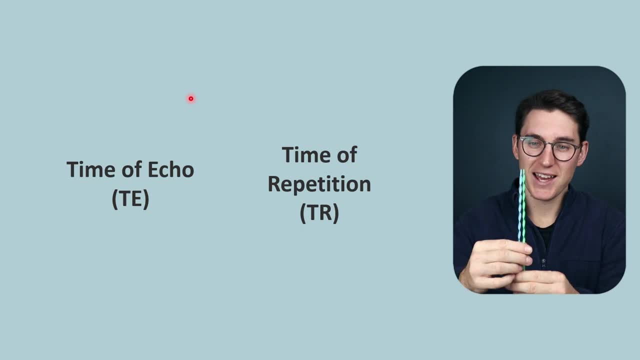 That signal gets lost as we get more and more out of phase. Now, the time of echo, is the time from that RF pulse, that 90 degree RF pulse, to the time that we actually measure the signal being generated by these tissues. Now, given more and more time, 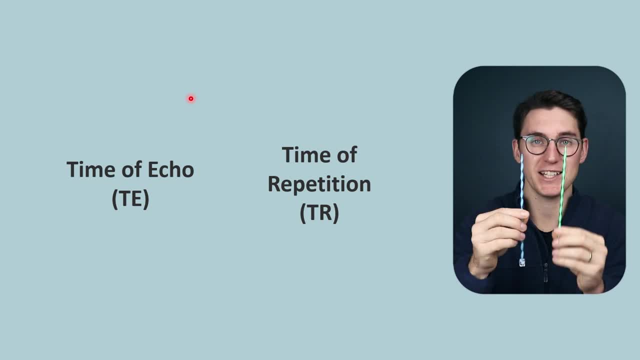 the phase, incoherence will become more and more. The difference between these two tissues will become more and more. So, as we wait a longer period of time, the difference between these two tissues will become more and more, But the signal will become less and less. 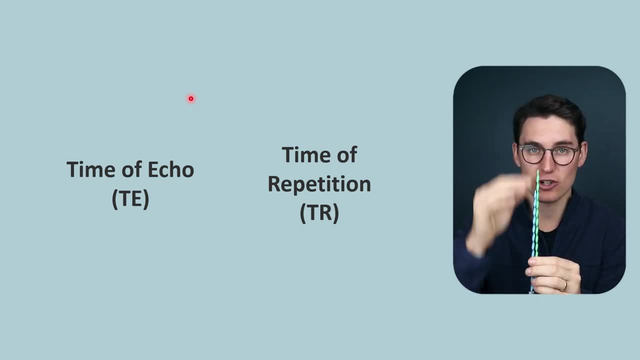 So it's a trade-off between getting good signal and getting contrast between these two tissues. Now that contrast is based on the loss of transverse magnetization. At the same time, both of these tissues are gaining longitudinal magnetization in the z-axis. 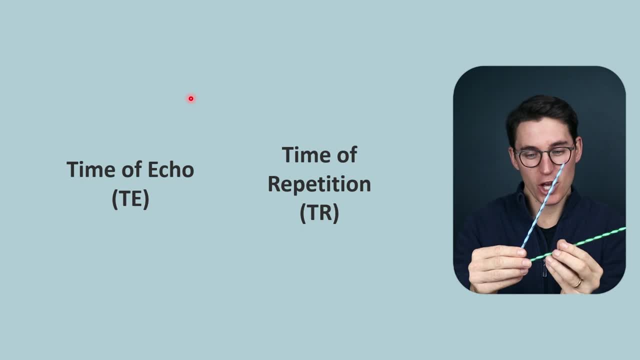 And if we wait a really long period of time we can see that they will gain their longitudinal magnetization at different rates, but if we wait long enough they will gain that full net longitudinal magnetization vector. We can then flip them again to 90 degrees with a second RF pulse. 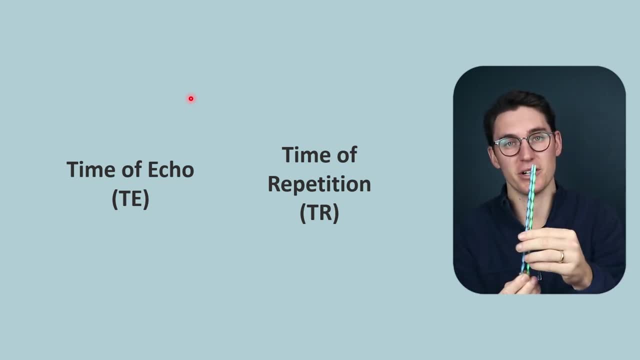 The time from that first RF pulse to the second RF pulse is what's known as the time of repetition or our TR time. If we wait a long period of time, flip it 90 degrees and then wait another period of time before measuring that signal. 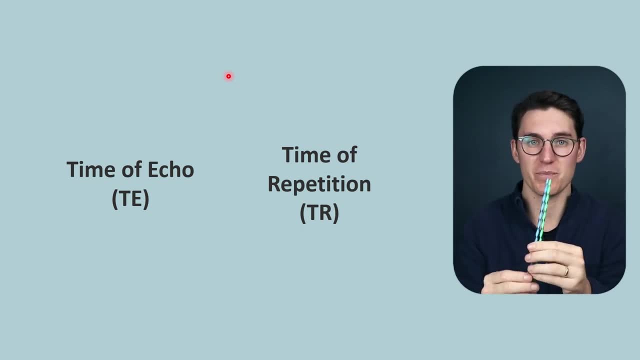 that time, to echo time from the RF pulse to when we measure the differences in signal, are going to be based on the loss of transverse magnetization. Now what happens? if we wait a short period of time, a short TR time, We'll see that longitudinal magnetization. 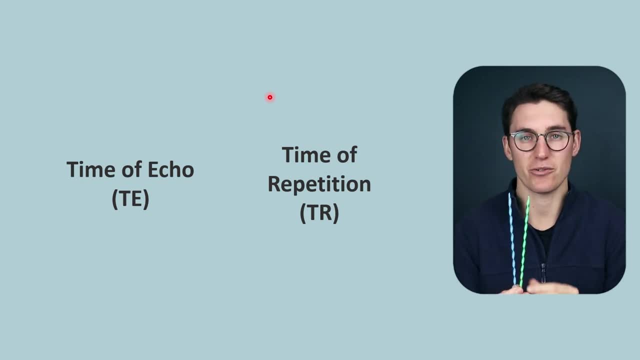 or longitudinal relaxation occurs at different rates. In fact, the longitudinal or T1, recovery happens much faster than it does in water. Now, if we wait a short period of time and don't allow the full net longitudinal magnetization or T1 recovery to happen, 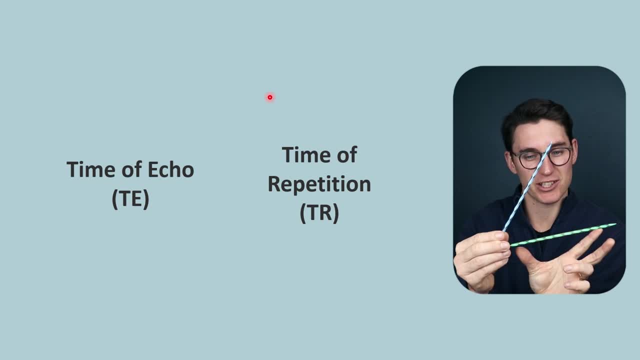 what we'll see is the longitudinal magnetization vector in fat is much longer than that of water. Now, when we apply a 90 degree RF pulse, the amount of transverse magnetization will only be equal to the amount of longitudinal recovery that has occurred. 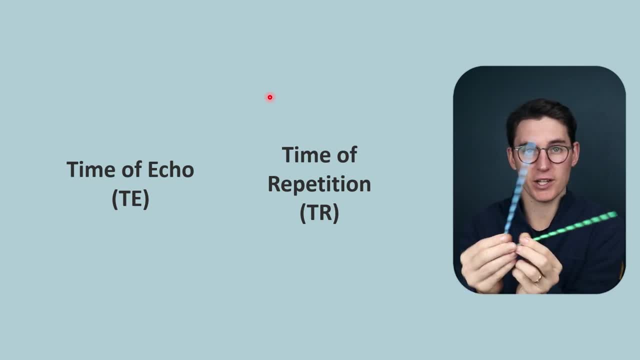 So our water will have a much smaller net magnetization in the transverse plane than the fat will. So when we flip this 90 degrees, this is what's going to happen. The signal that is being generated from fat is much more than the signal that's being generated from water. 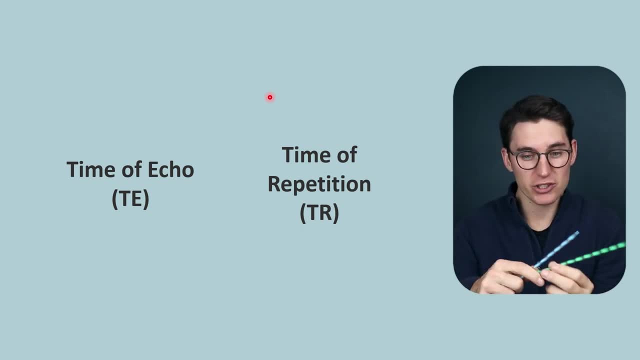 The difference that we are seeing here is because of that short time of repetition. It's because of the differences in longitudinal relaxation or the differences in T1 recovery. So when we make our time to repetition short, we're getting differences in longitudinal recovery or T1 differences. 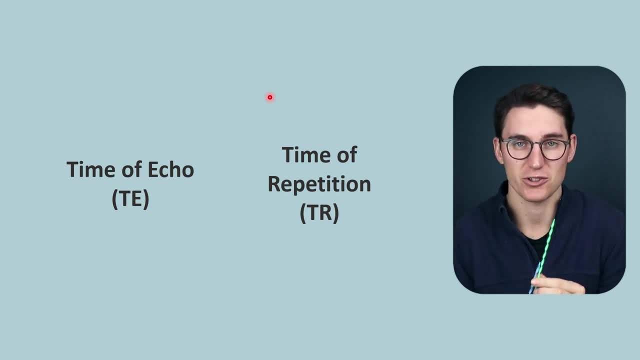 We are not measuring the T2 differences between these two tissues. Now, I know this is a really difficult concept and we have dedicated videos specifically looking at the types of relaxation and looking at TE and TR times. What I want to give you is an idea of 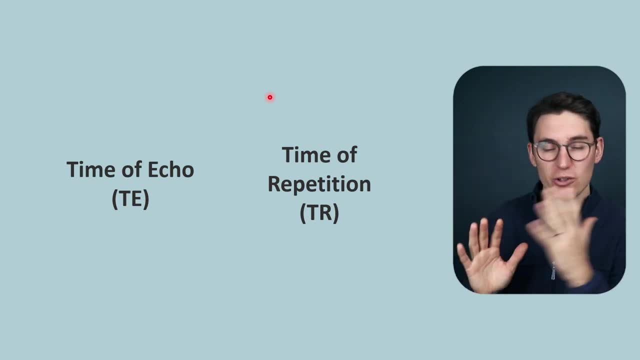 how we generate contrast in an image. and again, I'm just showing you the front cover of the puzzle that we are trying to create. You don't need to understand these concepts now, but it's useful to know where we're going in future lectures. 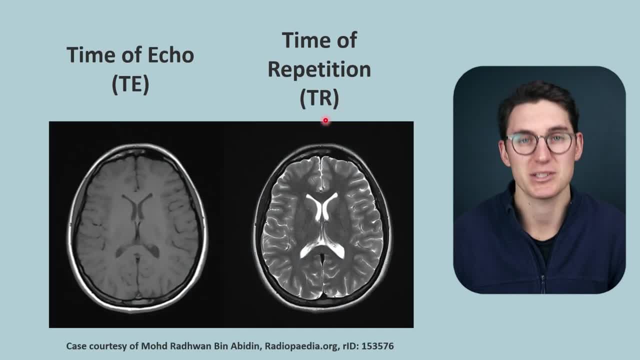 Now we can manipulate the TE and the TR times, as I've shown you now, to generate different contrast within our image. As I showed you in that example, with a short TR time the water lost its signal because it wasn't gaining its longitudinal relaxation. 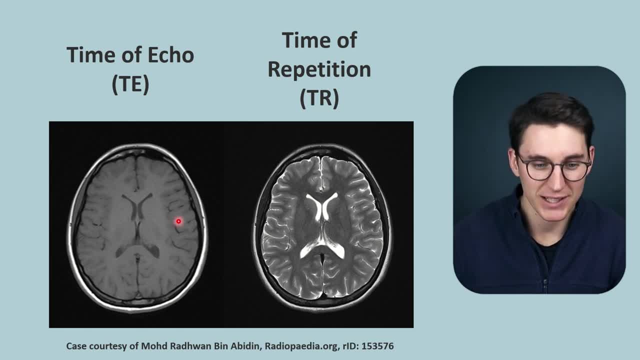 as fast as the fat was, And that's what's generating a T1 image where water, like our CSF, has a low signal and fat, like the subcutaneous fat here, has a high signal When we had a long time to repetition. 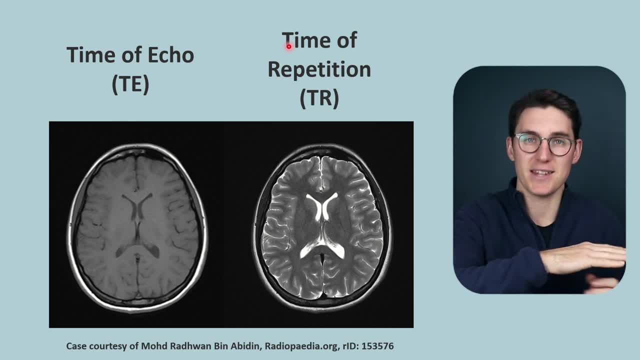 we allowed all of those tissues to fully regain their magnetization in the longitudinal plane before flipping them into the 90 degrees and then having an echo time that measured that transverse magnetization. That's what generates a T2 image, where the differences between water and fat now 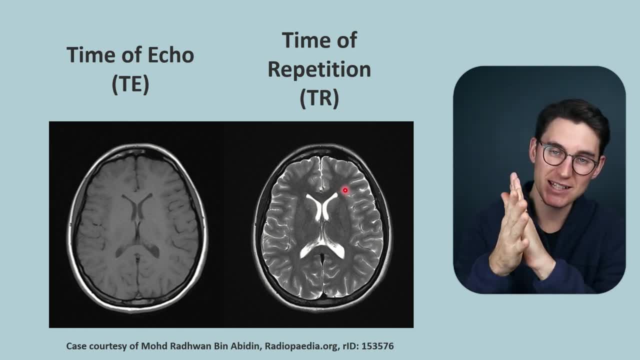 come from the differences in the rate at which they de-phase in the transverse plane. Water takes a very long time to de-phase and the signal remains high in the transverse plane, Unlike fat, which, because of the spin-spin interactions that we're going to look at in a future talk. 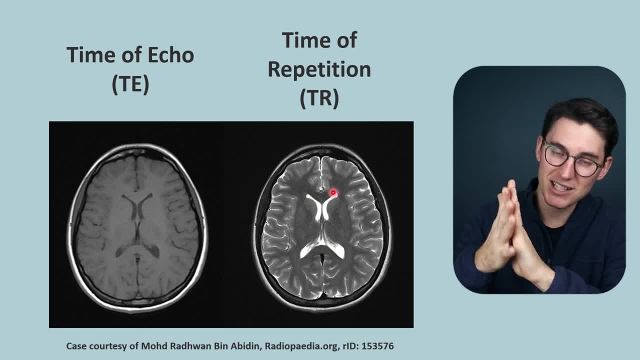 reduces the transverse magnetization signal because fat de-phases relatively quickly compared to water And we can see we get dark signal in the fat-coated axons in our white matter. we get bright signal in the water in our CSF. 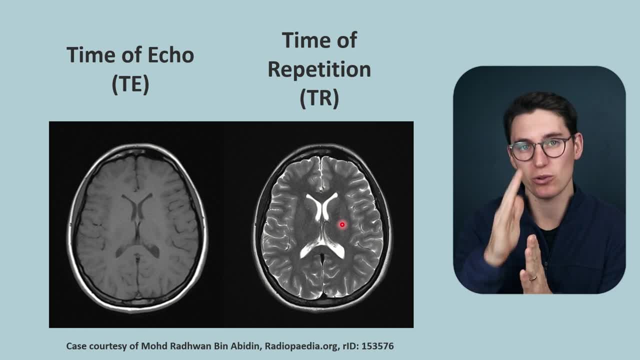 because of the differences in the T2 relaxation or the free induction decay between those two tissues. Now the way in which we actually generate these images is more complicated than what we covered here, but the underlying principle will always come back to the time of echo and the time of repetition. 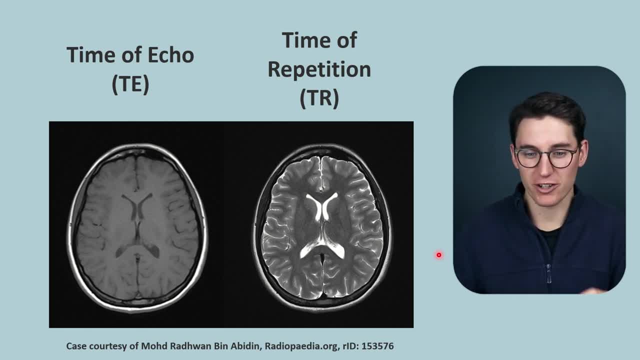 We still need to look at how we exactly go about localizing the different signals within the patient, how we select certain slices along the patient and then how we encode the different X and Y axis components of our image, And in order to do this, we use what is known as. 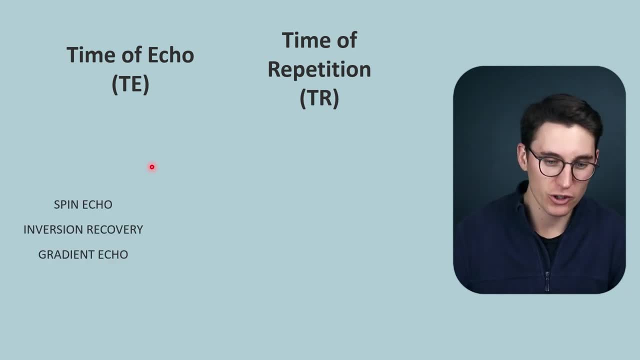 different pulse sequences and in this module we're going to look at the main pulse sequences: the spin echo sequence, the inversion recovery sequence, as well as gradient echo sequences. We will then expand on these different sequences, looking at more advanced imaging techniques. 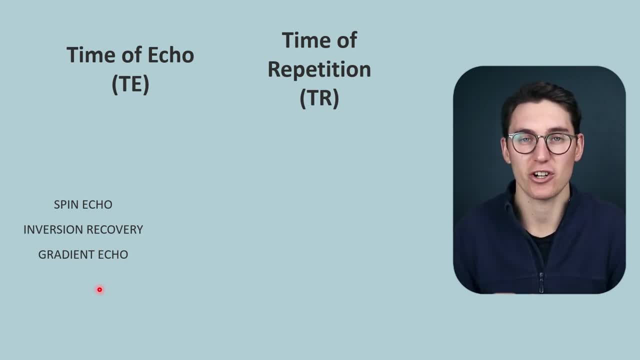 We'll also look at MR spectroscopy, as well as different types of angiography in MRI imaging. We'll end off the module by looking at different types of MRI artifacts, as well as image quality and safety within MRI imaging. Now, when we are generating signals.